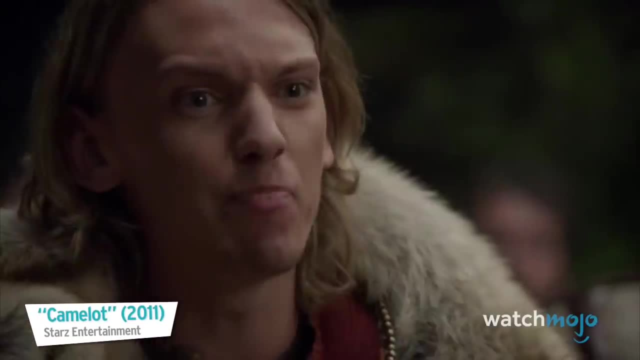 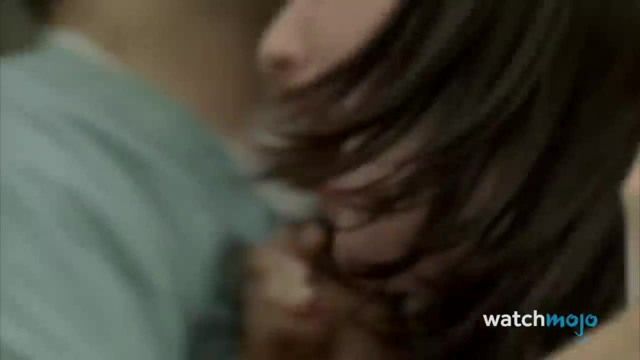 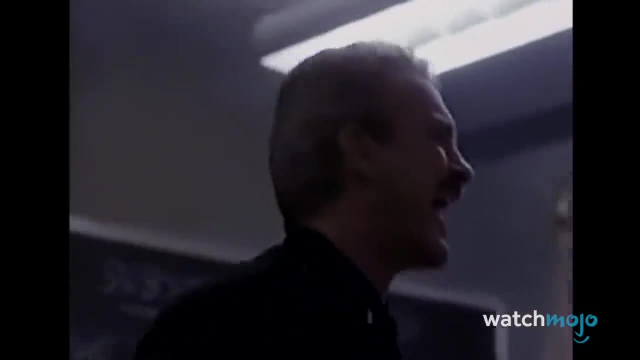 And you will pledge your allegiance to me or suffer for it. Understand that you bearded fool. As TV slowly ventures further into big-budget productions, it's only natural that a few fall flat. Welcome to WatchMojocom. and today we're counting down our picks for the top 10 most expensive TV flops ever. 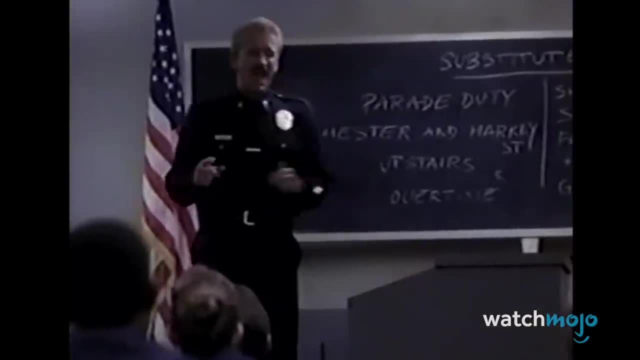 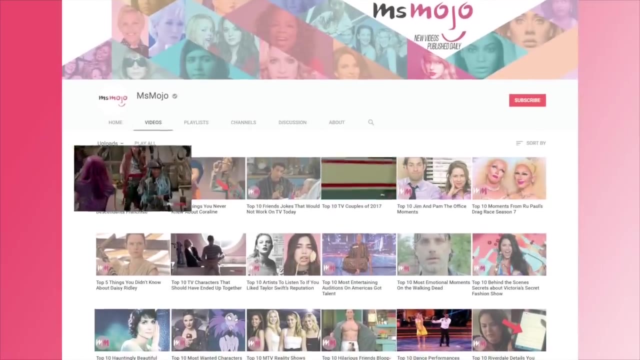 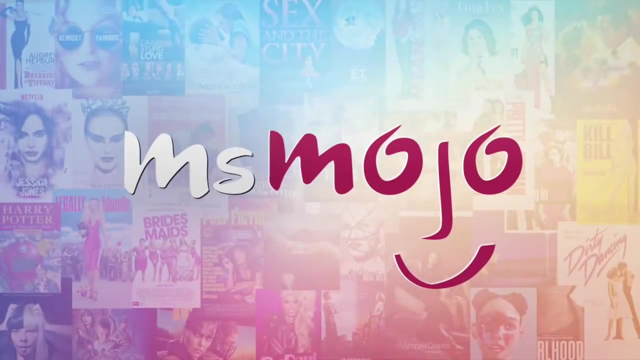 Play it tough but play it safe, And let's be careful out there. If you like this video, then you'll love the original content over at our sister channel, Ms Mojo, your source for all things pop culture, celebrity and entertainment. 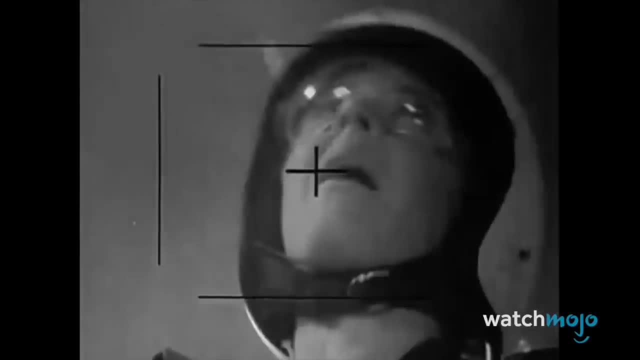 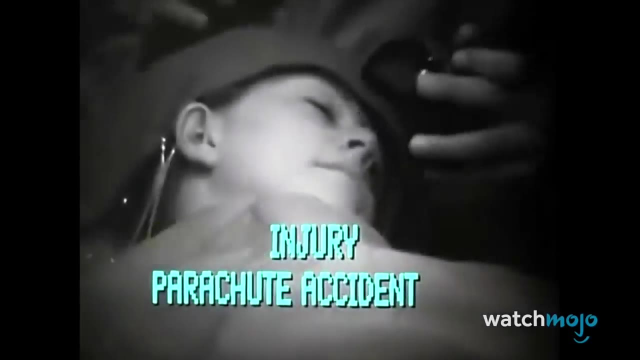 For this list. we're discussing some of the biggest flops in television history and ranking them based on the severity of their failures. Now we're not saying these shows are bad- In fact, many of them are quite good- We're only stating that they failed to find a mainstream audience. 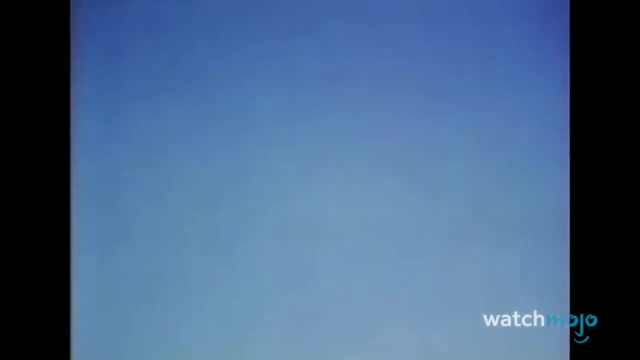 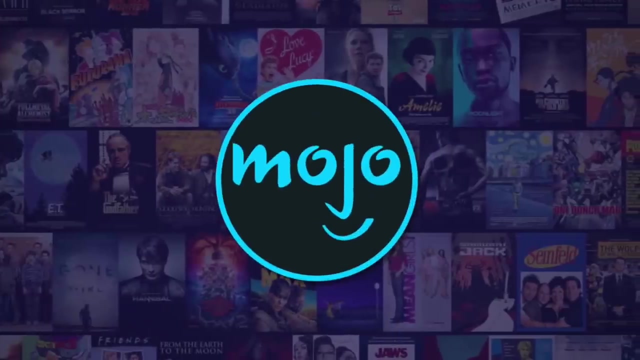 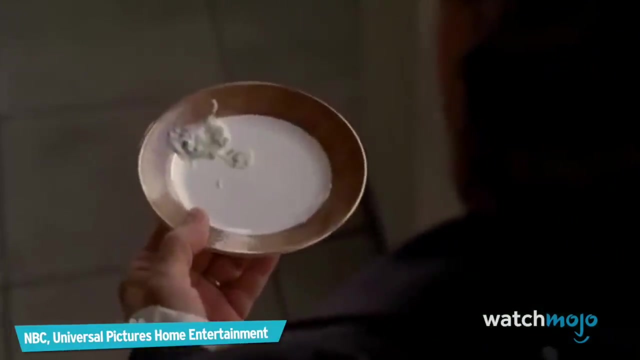 and were swiftly cancelled, losing their studios a ton of money in the process. 10. Kings- Kings was set to be NBC's great drama. It was based on a biblical story. it starred the incredible Ian McShane, fresh off his revolutionary performance as Al Swearengen on Deadwood. 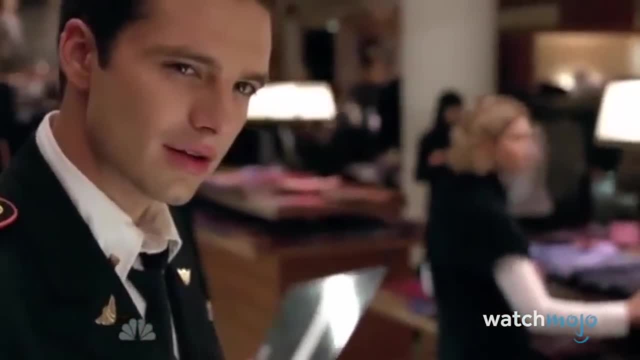 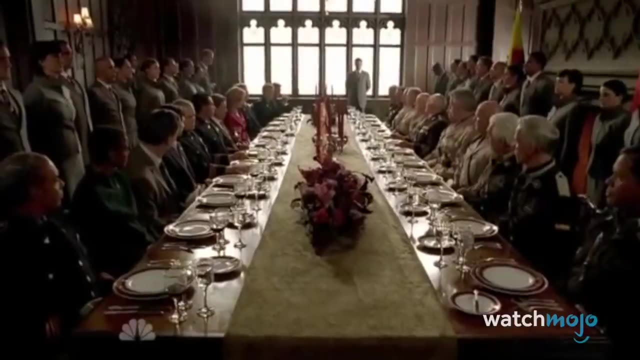 and the studio reportedly put up a whopping $10 million for its pilot. The subsequent episodes weren't much cheaper, most of them coming in with a $4 million bill, Just like in the movie. Judging by those numbers, we can assume that the 13 episodes of Kings. 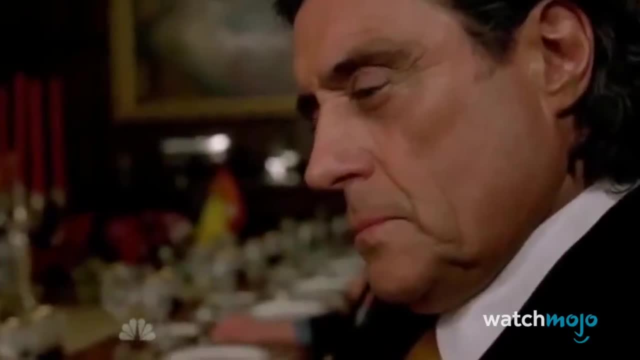 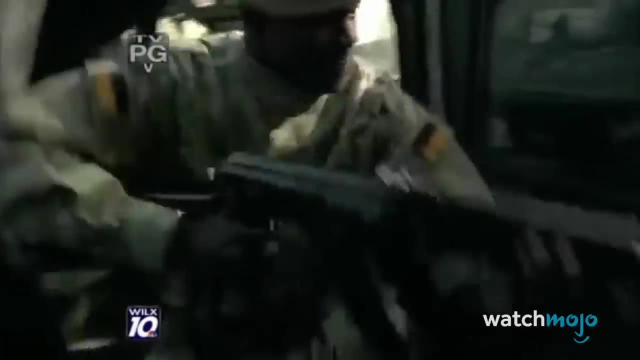 including its two-part pilot, cost well over $50 million to produce. However, the show received middling reviews and viewers quickly dropped off after the first couple of episodes, resulting in Kings' swift cancellation. Don't go Stop. we're all out of here. 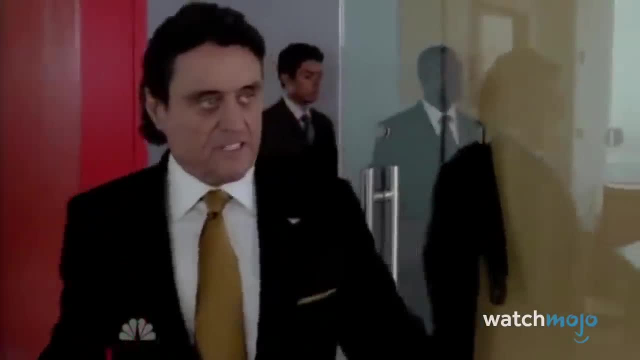 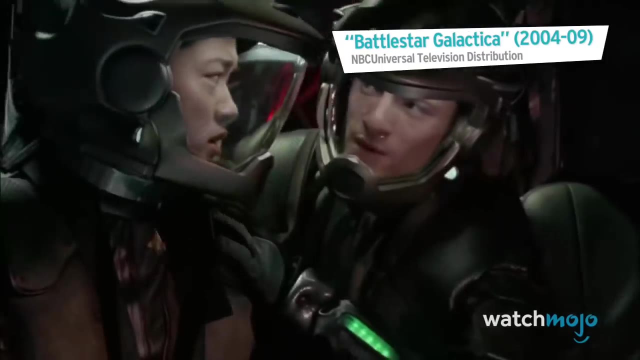 Get your hands off me. please. Talk about a short reign. It's treason what you've done. 9. Battlestar Galactica. Before getting a new and enduring lease on life, the Battlestar Galactica franchise kicked off with a TV series in the late 1970s. that rode the sci-fi popularity wave of the first Star Wars film. Right here you creeps. And like most convincing science fiction, it wasn't cheap to produce. Each episode cost about a million dollars to produce, or just under $4 million in today's dollars. 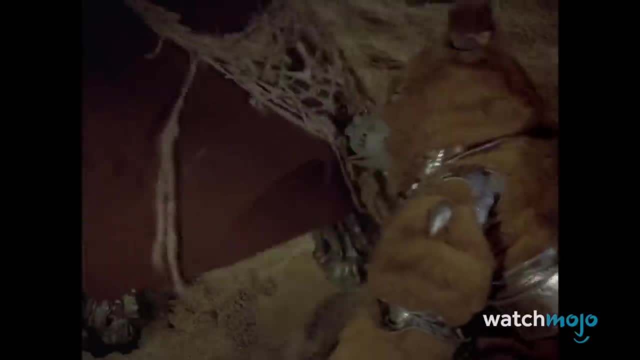 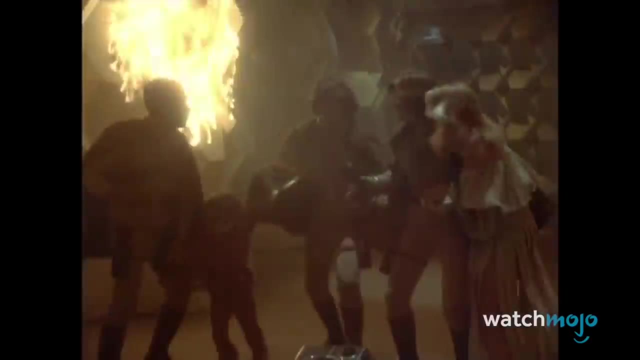 And while Battlestar Galactica initially saw success, it quickly sunk in the ratings. when CBS moved its hit show All in the Family to the same time slot, ABC cancelled the show after one season, leading to protests and, unfortunately, 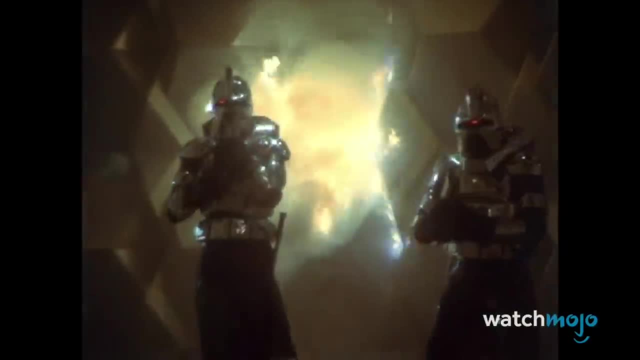 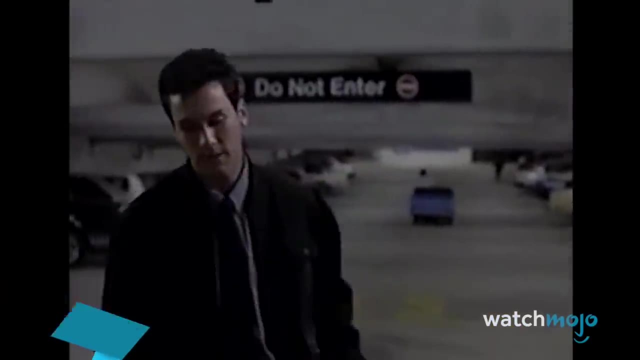 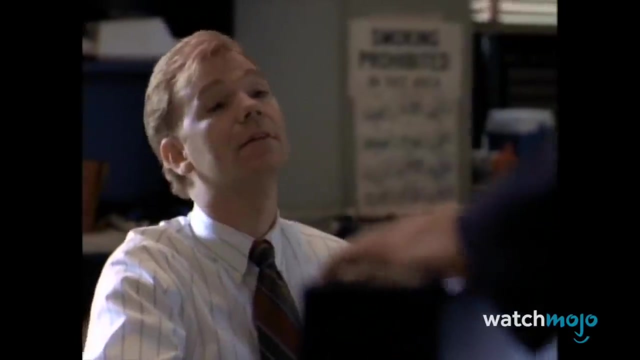 the suicide of one fan, Oh frick 8.. Cop Rock. Mom always told me be nice to strangers. Cop shows were big business in the 80s and 90s Series, like Hill Street Blues and NYPD Blue. both garnered critical acclaim. 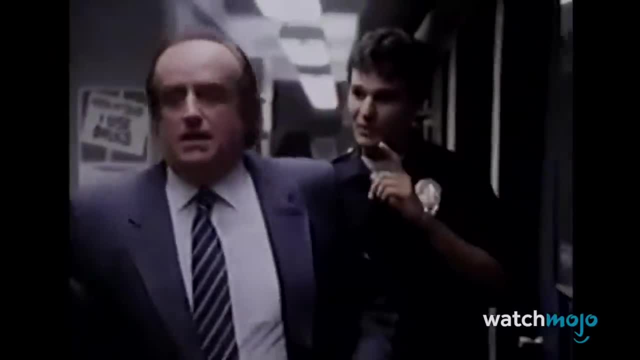 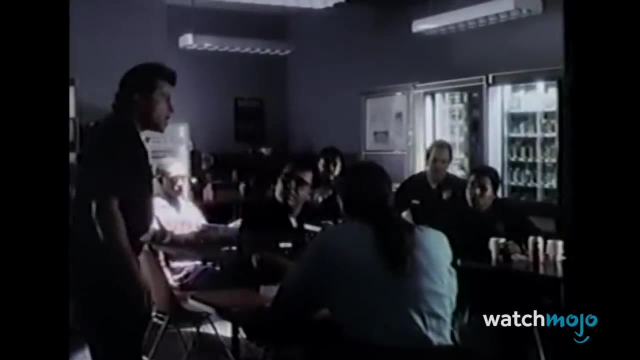 and devoted audiences. Cop Rock, a musical cop drama- yep, you heard that right- unfortunately didn't fare as well. It's often considered one of the worst dramas of all time and it unsurprisingly didn't garner much of an audience. 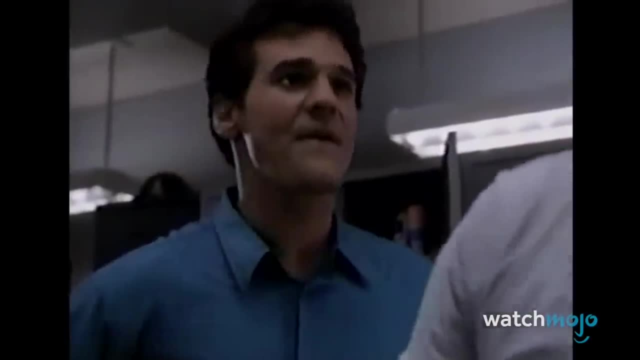 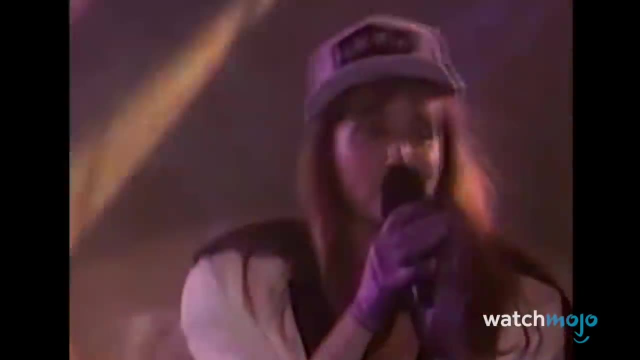 Each episode cost almost $2 million to produce, or just under $4 million today. but despite its lavish production, its bizarre concept was just too much to handle. ABC cancelled the show after just 11 episodes and Cop Rock was deemed one of the biggest TV failures of the decade. 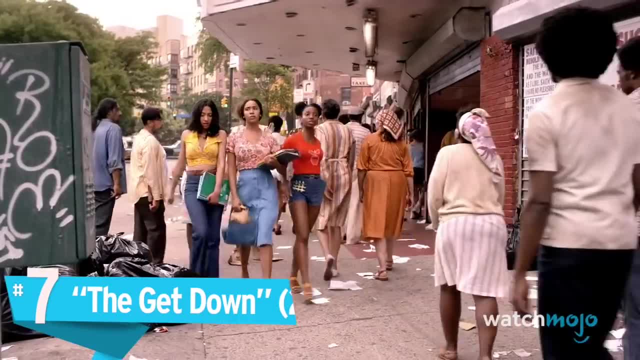 and Cop Rock was deemed one of the biggest TV failures of the decade. and Cop Rock was deemed one of the biggest TV failures of the decade. Sorry, Netflix, they can't all be winners. The Get Down was a massive production from Baz Luhrmann. the artistic visionary behind gorgeous productions like Romeo and Juliet, Moulin Rouge and The Great Gatsby. The Get Down was a massive production from Baz Luhrmann. Netflix originally planned for the show to cost $11 million per episode, or about $120 million for the season. But the budget ended up ballooning as high as $16 million an episode. The final budget was estimated to be somewhere between $180 and $200 million- about as much as a Marvel production. Unfortunately, the gamble didn't pay off and Netflix was forced to cancel the show after one season. 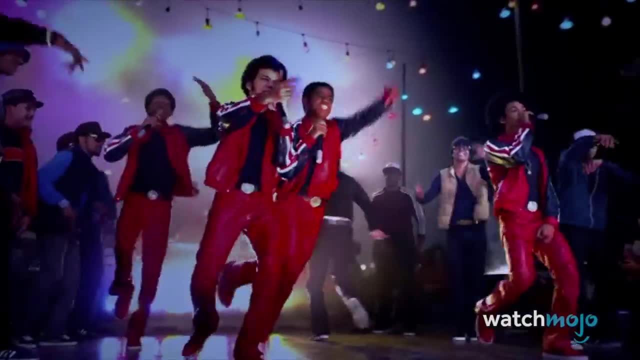 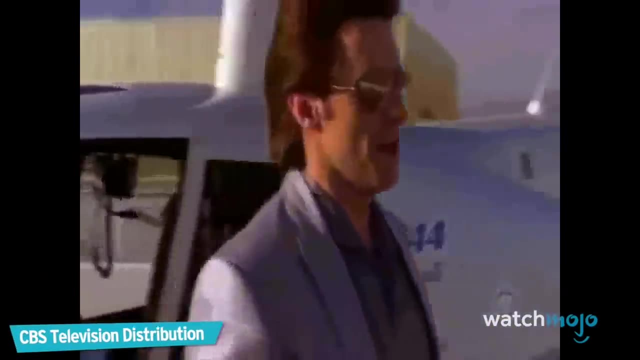 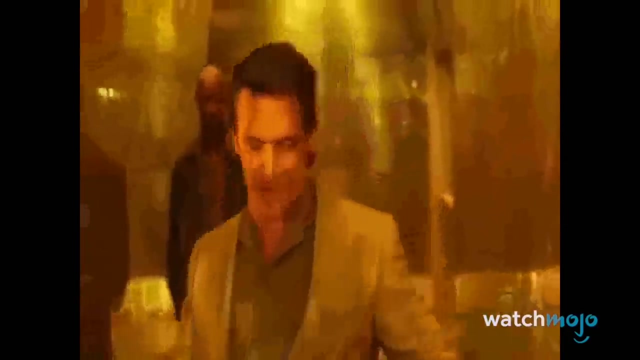 due to its low viewership and exorbitant costs. Number 6. Viva Laughlin. Viva Laughlin was an ambitious project from CBS. Hugh Jackman starred and served as executive producer, and the pilot episode alone cost nearly $7 million to produce. 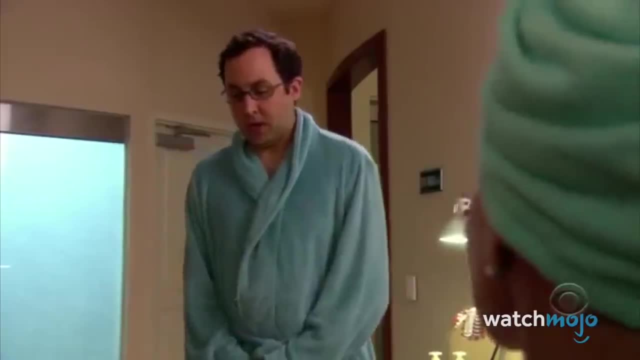 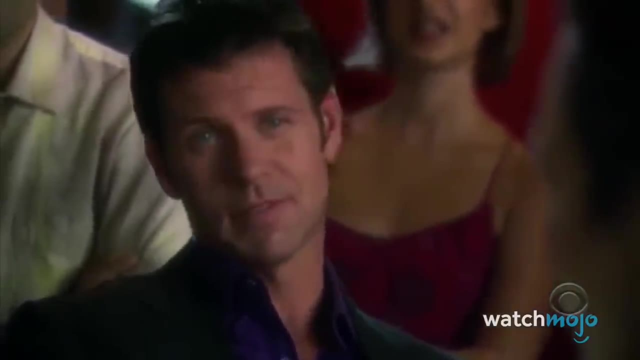 However, the show was absolutely roasted by critics, with one writer from the New York Times questioning whether it could possibly be a contender for the worst show of all time. That's rough. The viewers seemed to agree, as the show was quickly cancelled. 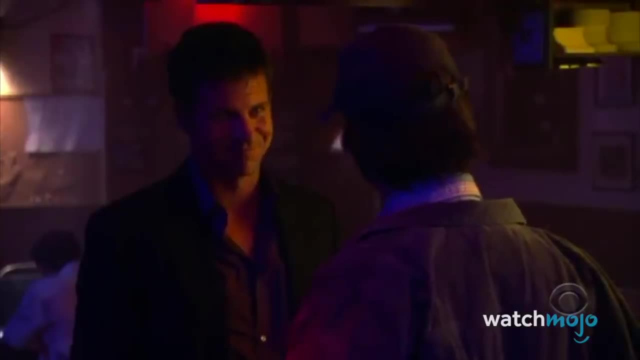 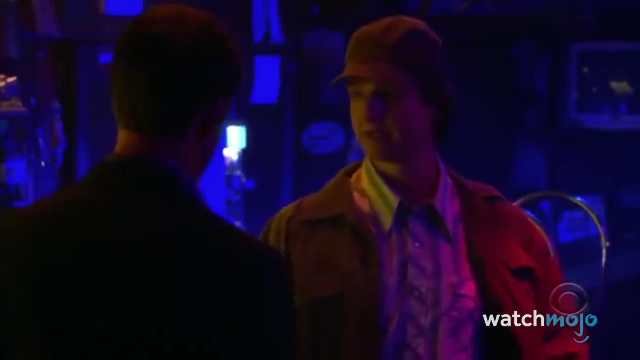 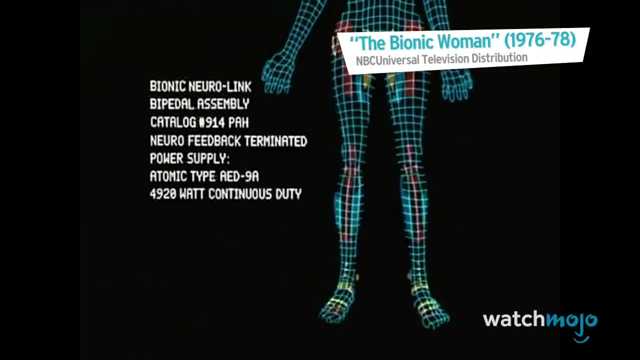 And we mean quickly. The show received the axe after just two episodes, leaving five produced episodes unaired. Now that's what we call a bomb Number 5.. Bionic Woman. The Bionic Woman was a hit in the 70s. 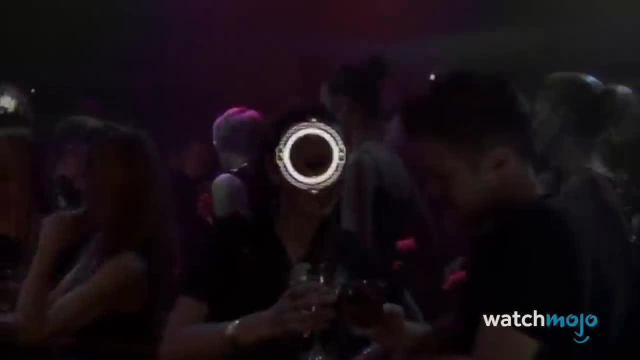 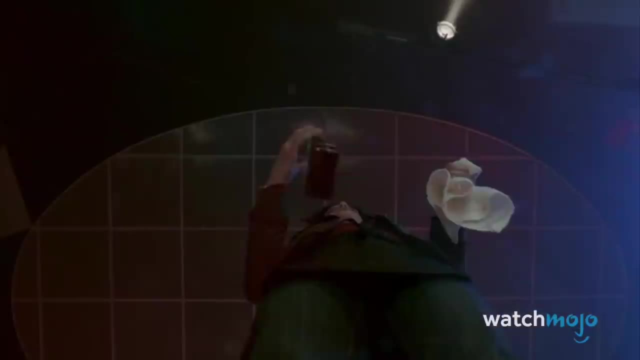 so naturally, it was bound to get the remake treatment. The reboot debuted on NBC in 2007,, but the critics absolutely didn't. NBC despised it and, despite respectable viewership numbers, the writer's strike of 2007 put an end to the show's production. after just eight episodes. This spelled disaster for NBC, as each episode of the show reportedly cost around $6 million to produce and the network spent $15 million on marketing. Judging by those numbers, NBC spent around $60 million on a show that was cancelled. 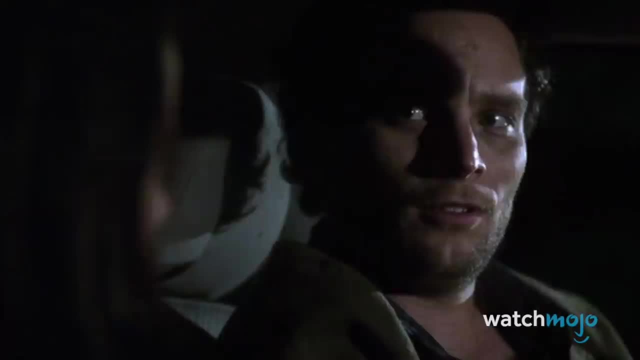 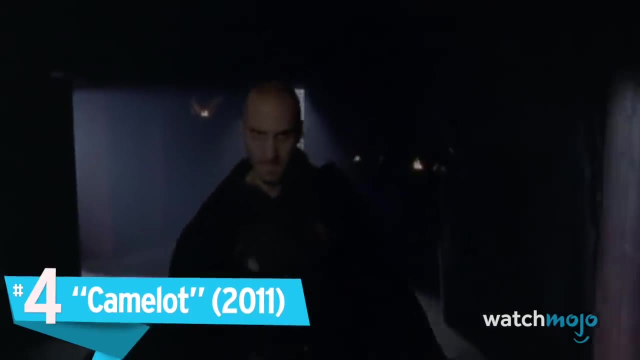 after just eight episodes, Not exactly a good return on investment. Do you really have x-ray vision? Yeah, Yeah, I do. Number 4. Camelot. Camelot was another star's attempt at a sword-and-sandal drama after Spartacus proved to be a big hit. 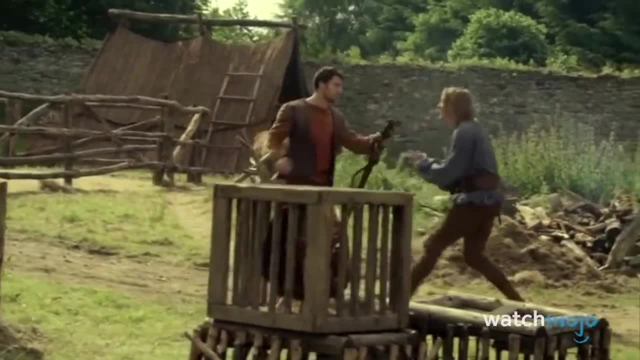 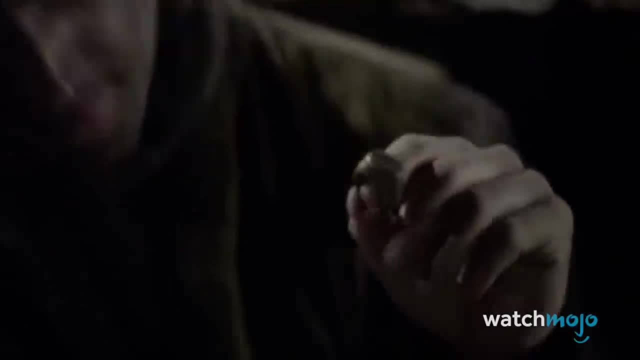 Spartacus. this was not. Oh shut up, Please just shut up. The show was run by Torchwood and the Tudors' alums, Chris Chibnall and Michael Hurst respectively, and it starred Joseph Fiennes and Ava Greene. 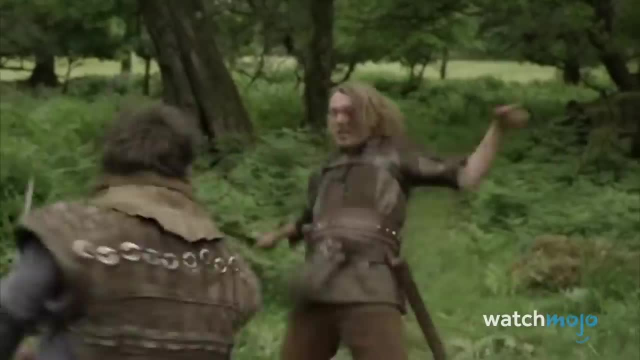 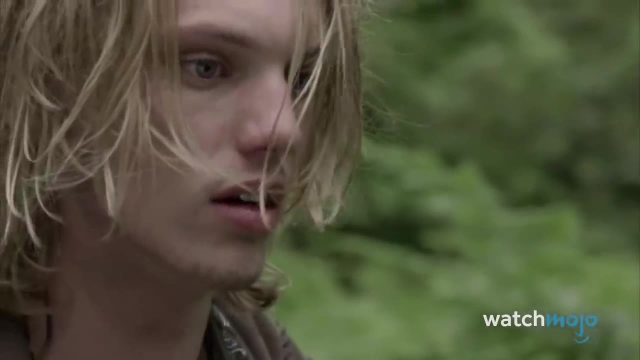 If you think this sounds expensive, it was. Each episode cost around $7 million to produce and, with 10 aired episodes, it's assumed that STARS pumped about $70 million into Camelot. We're here when they find him. 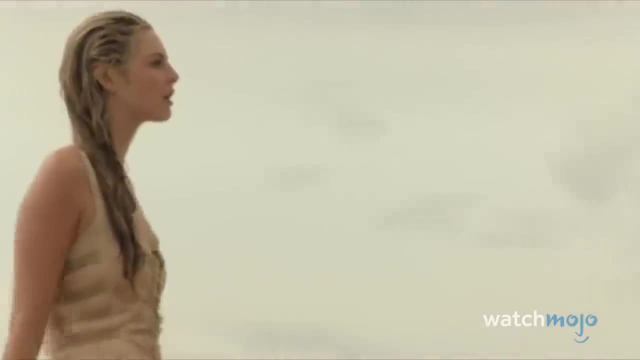 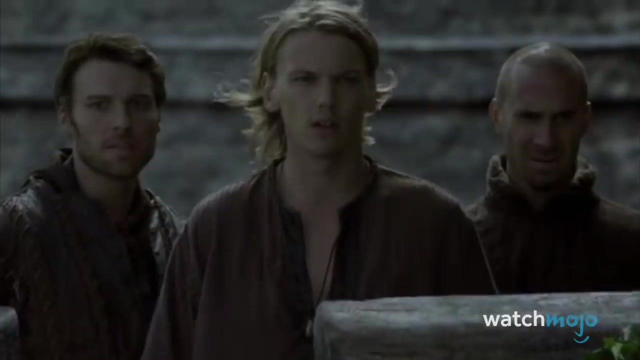 He won't live to be king. However, the show was criticized for being dull and silly and, despite the premiere being the highest-rated pilot in STARS history, it was cancelled after 10 episodes due to scheduling conflicts with the cast. 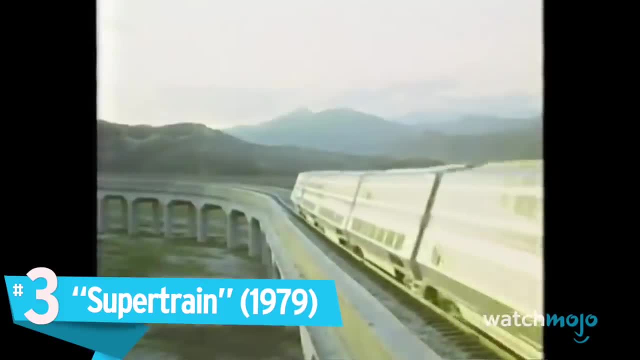 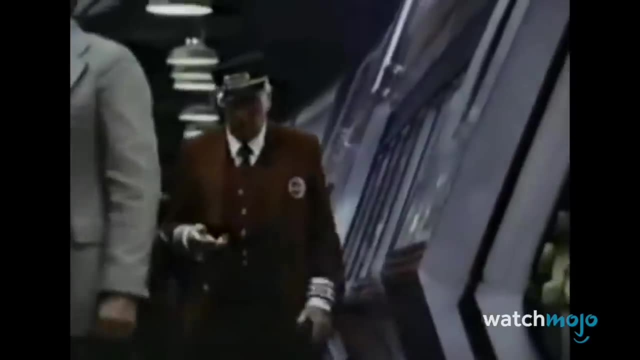 What do we do now? Number 3. Super Train. Super Train was a great show. It was a great show. Super Train was a great show. Super Train is known for being one of the biggest laughs in television history and unfortunately, it wasn't a comedy. 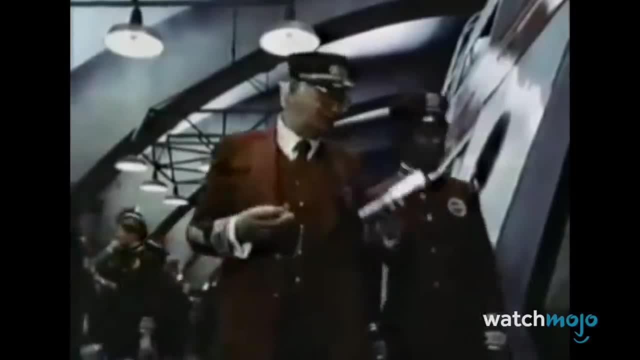 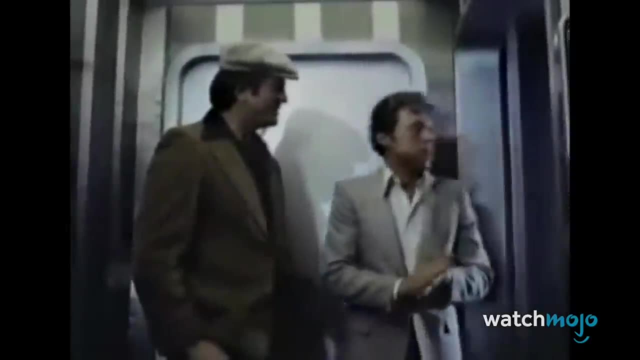 Engine room Super Train is ready to depart. It's often ranked in worst TV show lists, and it was a massive commercial failure the likes of which had never yet been seen. You sure about that, huh, While exact numbers are hard to come by, 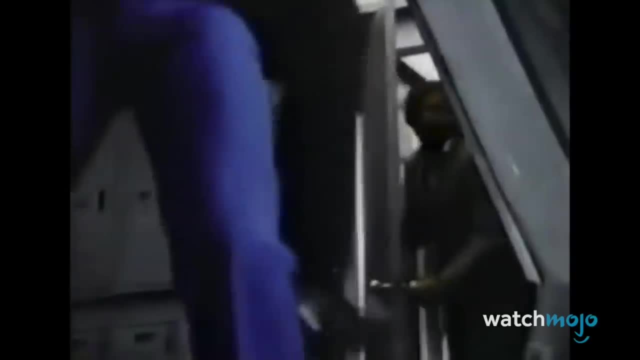 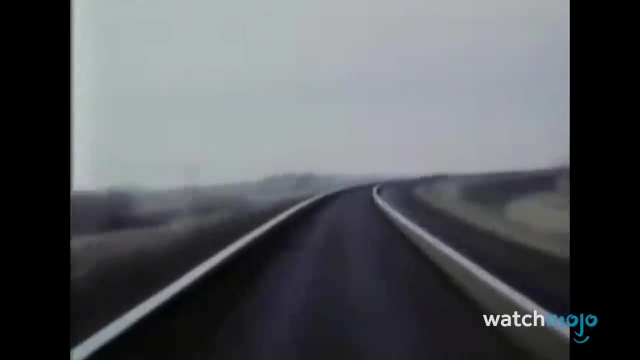 Super Train is considered the most expensive American show ever produced at the time, and NBC put a massive amount of money behind its marketing. However, the show's poor quality resulted in low viewership and it was cancelled after just three months and nine episodes. 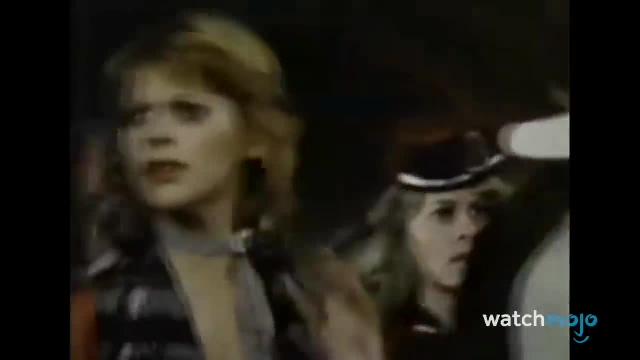 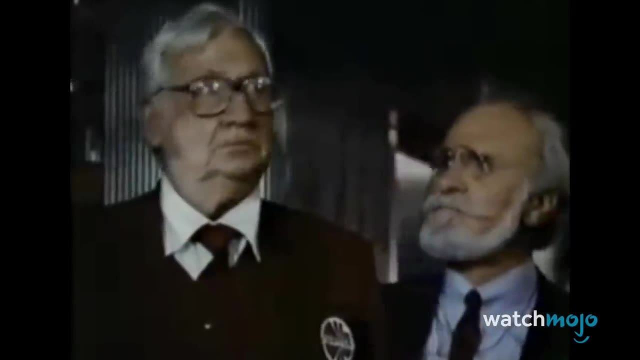 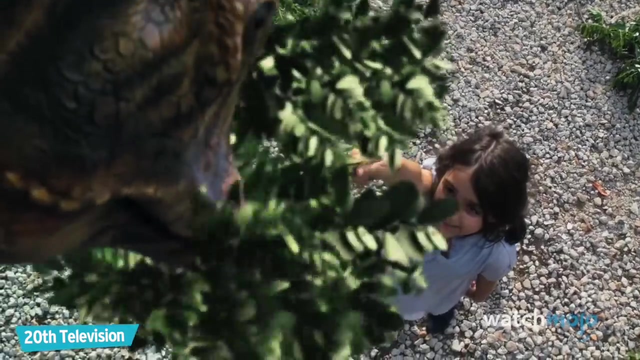 NBC wasn't able to recover its enormous losses and the network nearly went bankrupt. I thought we were given assurances that that window was indestructible. Number 2. Terra Nova. Science fiction's always tricky to produce. It costs a lot of money to make convincingly.